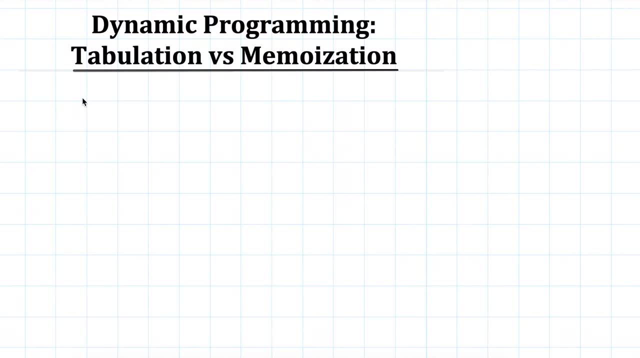 Dynamic programming is an optimization algorithm over recursive solution. So if some recursive solution solves its sub-problems multiple times, dynamic programming comes in handy and brings down time from exponential order to polynomial order. So the main objective is that once we have solved any sub-problem, we don't need to re-solve the same problem. 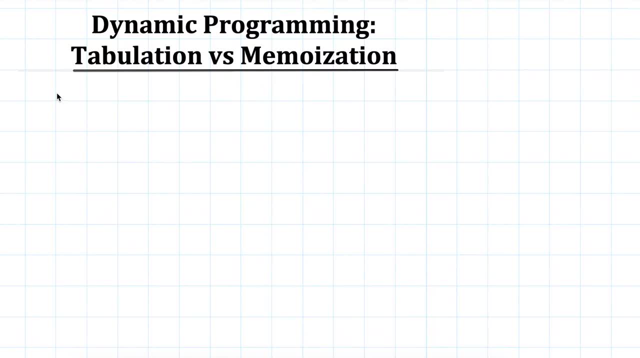 again and again, multiple times. So somehow we need to store those values. So once we calculate any value, we need some mechanism to store. And we have two ways to store those values. So we follow either tabulation, which is solving the problem bottom-up, or we can. 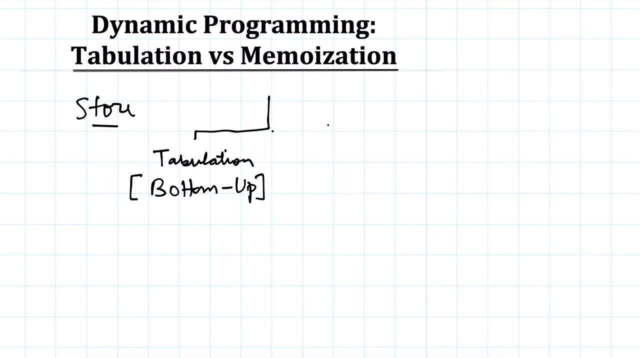 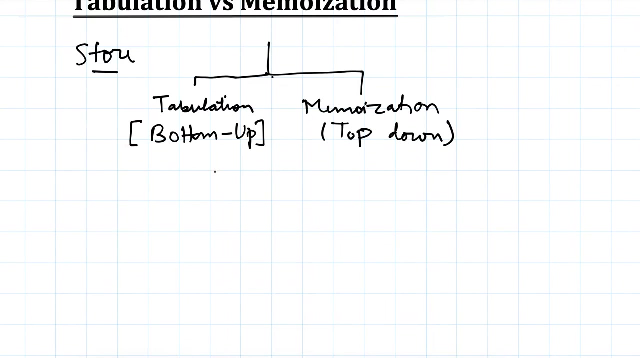 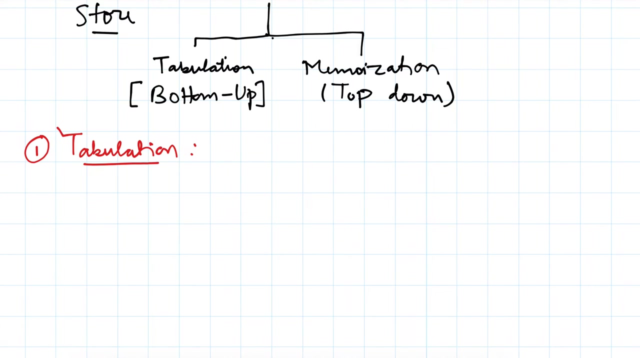 call it top-down, or the other is top-down, which we call memoization. So this is top-down. So now we will see what is the difference between the two. So first let's look at top-down Tabulation method, that is, bottom-up approach. So here we start from the bottom, or we call 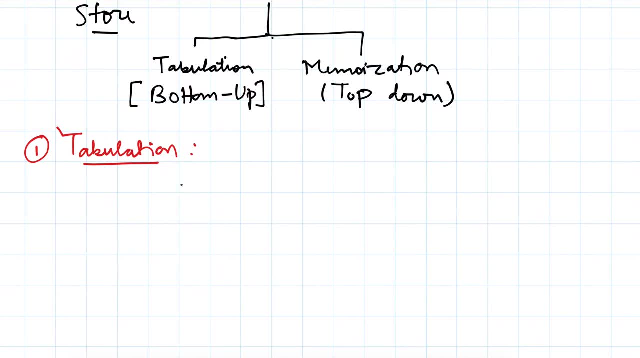 that the base case. So we can have some straight transition relationship, like we have some base state 0. So we can have some straight transition relationship, like we have some base state 0. And from this base state you can go to 1.. It can be more, but for simplicity let's: 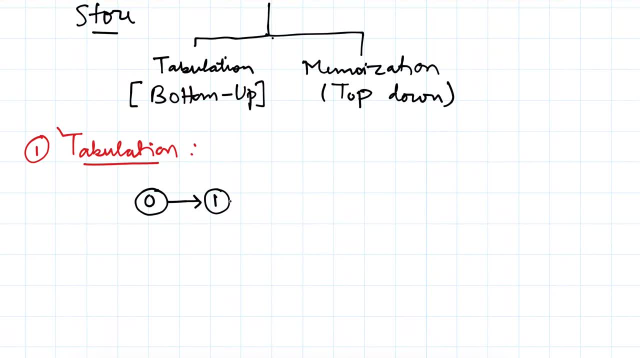 assume there is just one state where you can go to, From 1, you can go to state 2 and so on, And the topmost state is state n And this is your destination, And this is source, or we will call it base state, And this is destination state. So you first solve this. 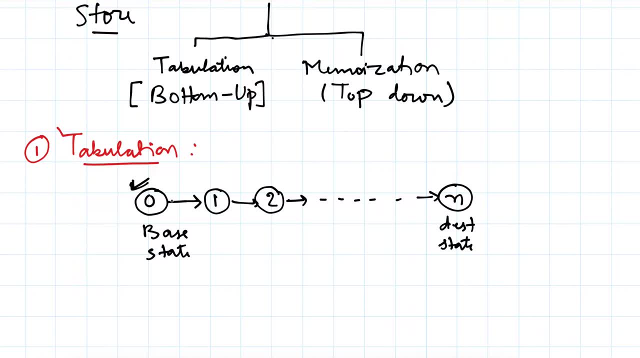 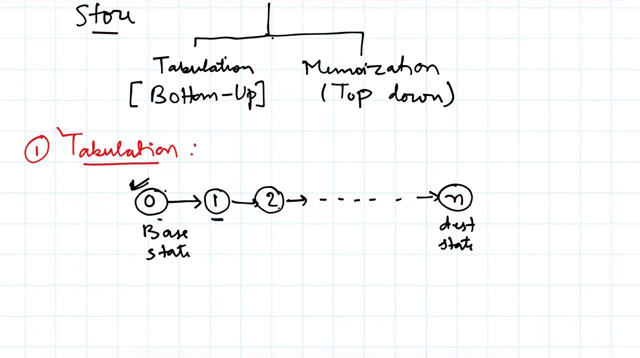 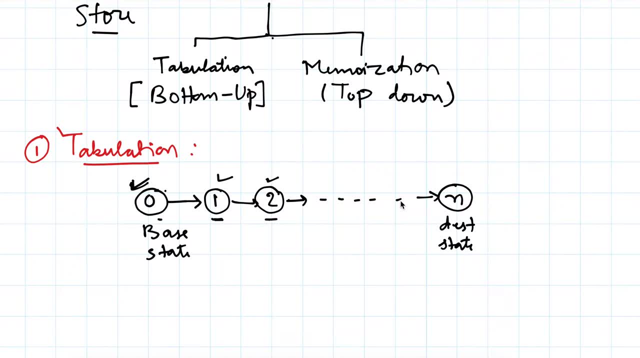 So we can use that value and solve state 2.. Similarly, here will be n minus 1th step state and after solving this, we will reach state n, And now we can solve this. So we start our transition from base state. 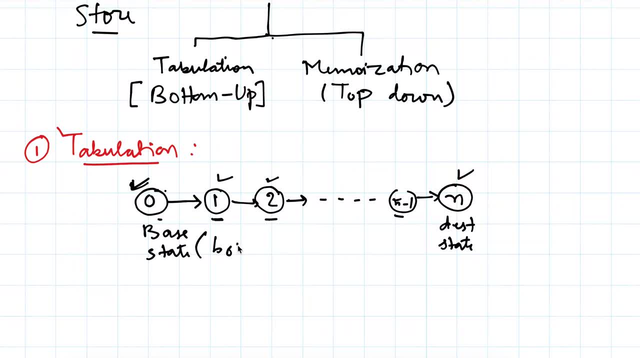 and we call that base state bottom and the destination state as up. this is the topmost state and we follow the state transition rule. so these are the state run in this state transition graph. you see that from 0 we can go to state 1, from 1 we can go to state 2. so this is called state transition relationship in. 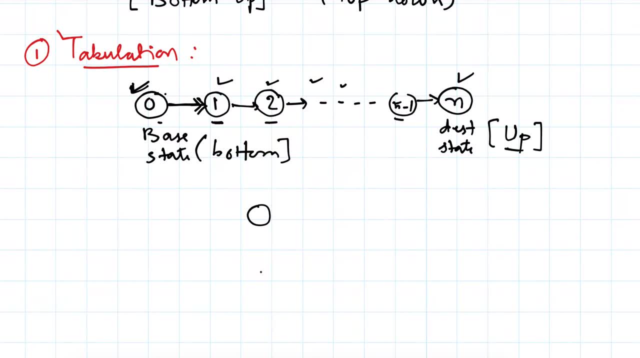 some complex graph you may have multiple nodes, like there is a transition possible from here and so on. so if this is destination state and maybe take one of these, this, as source state, then from source you can go to this state and from here you can go to this state. and there is other way you can move to here. 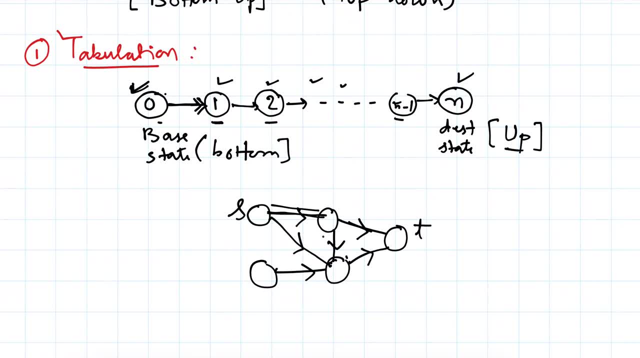 and then here. or, third way, go here, then come down, then go here, and if we look at the destination state, there are two possible ways to reach here, so that will be the other approach that we will see. so instead of moving from source to destination on the base state to destination, we start from the top and 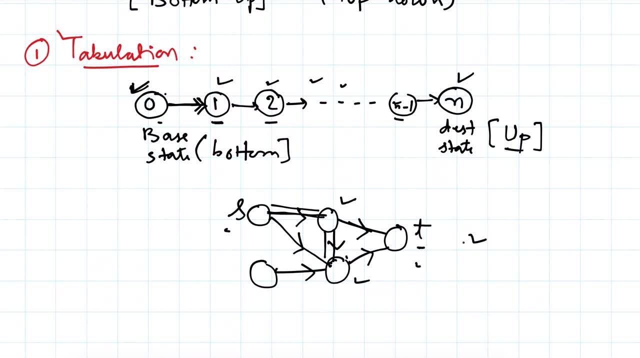 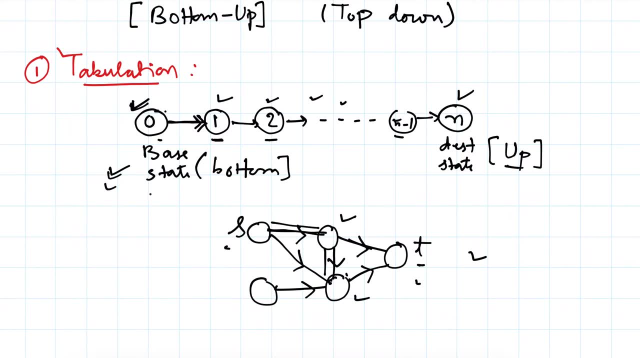 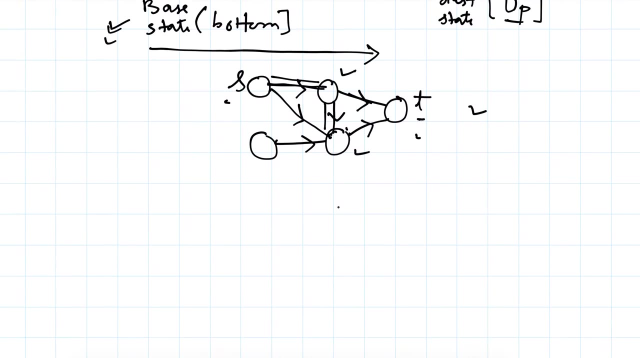 see where, from where we can reach. that will be the other state, the other approach, the memoization approach. so so this is tabulation approach, where we start from base and solve it and then move to towards higher states and ultimately we will reach the destination state or topmost state. that is the 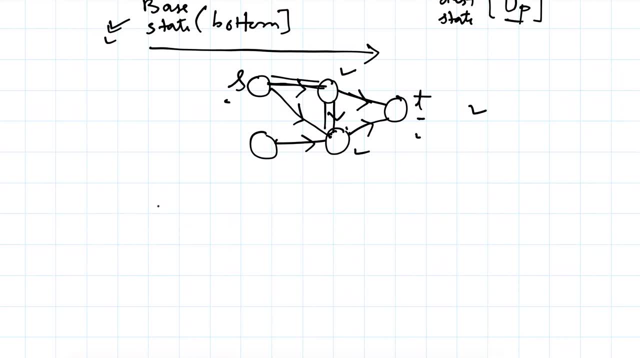 desired state for which we want to solve. so I will give one small example here and then I will show you how to solve it. so I will give one small example of factorial function. so we want to find the factorial of X. then what we do? we take one array, so your name of air and function are same. so let's take some. 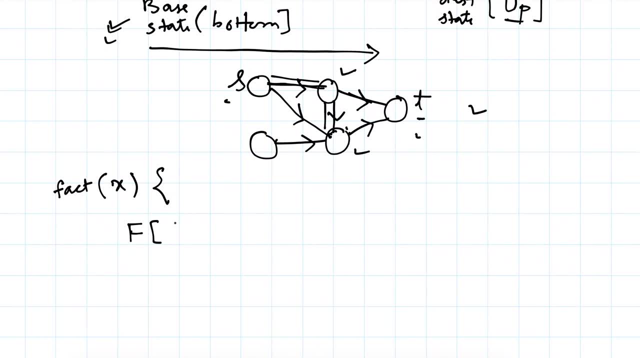 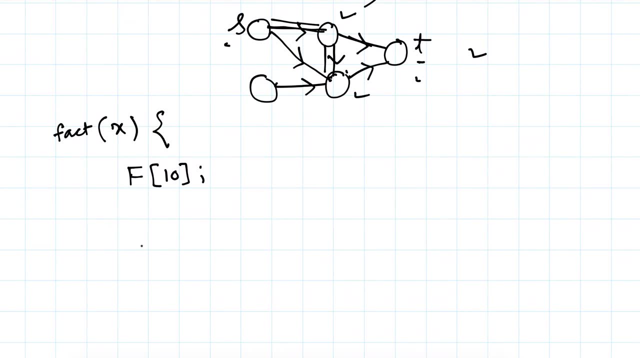 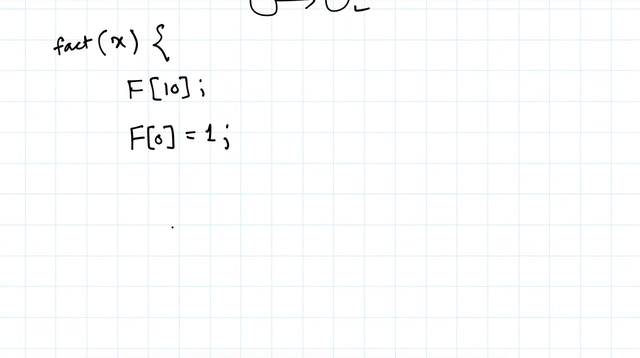 different name and then we can initialize: the base case that is, factorial of 0, is equal to 1, so this is our base case, or base state, and then for I, equal to 1. so so this is X, because we want to find the factorial of X. 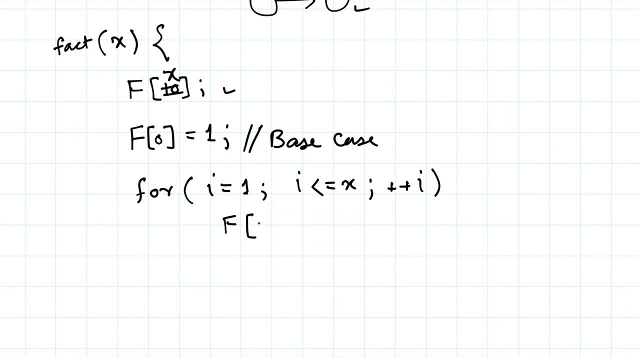 and then. so, as for X and 1, this type of thing is 650 times 150 plus X is equal to 1. so the factorial of I is factorial of I minus 1, x, that number, but we're starting from 1.. So we will need f of zero, which we have initialized base case. 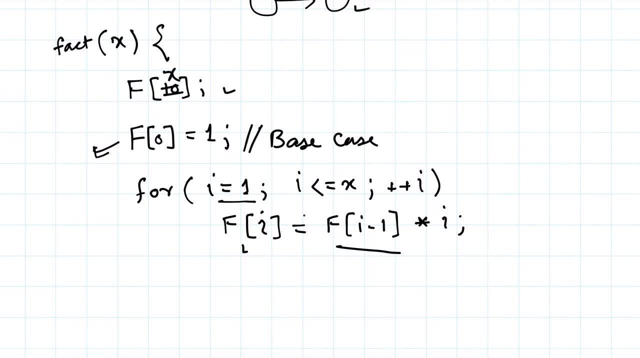 so force it will find to say: to син x L minus i minus 1 V times 5, by that number find f1, then f2, until it reaches X, and then we can return fx. so here no problem is solved. 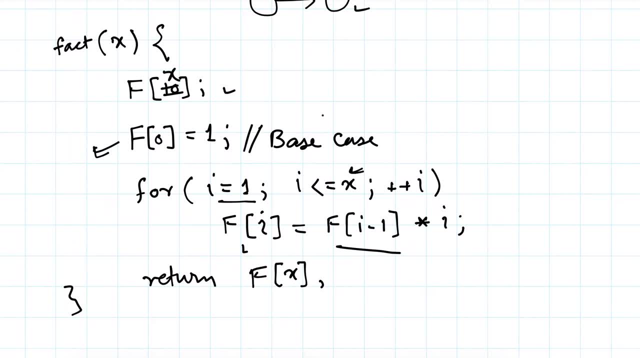 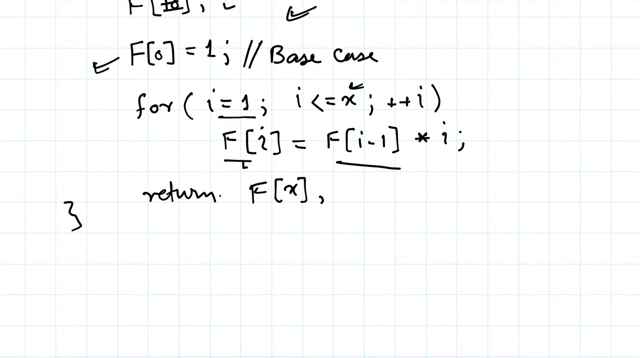 solved twice and all the base cases are required, like we cannot find f10 without knowing f9, and we cannot find f9 without knowing f8, and so on. so we start from the base itself and move towards the top, solving every problem just once, and we are storing the value in this f array. so 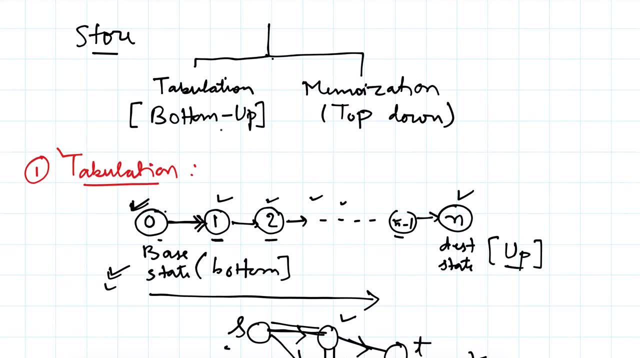 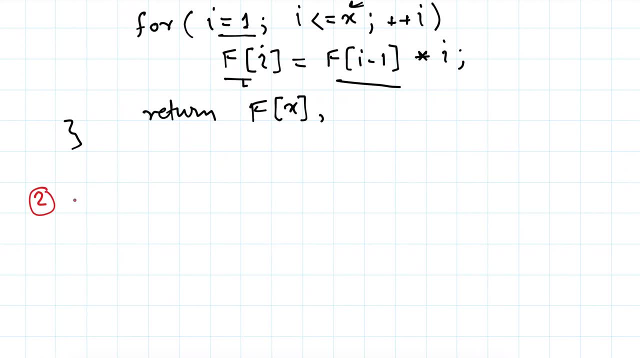 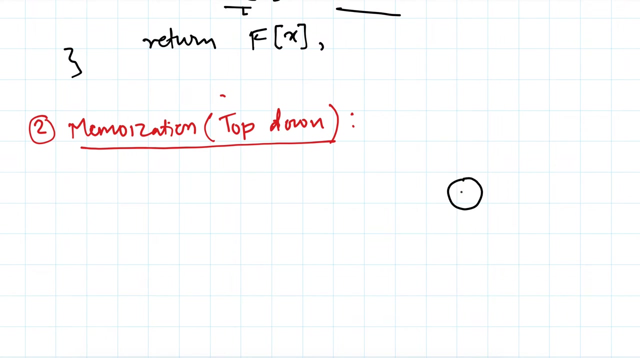 this is the bottom-up approach, or tabulation of approach. now let's look at the second approach, and this is called top-down. so here we can see the same diagram like: if I want the value of state n, which depends on state n minus one, so it will call its. 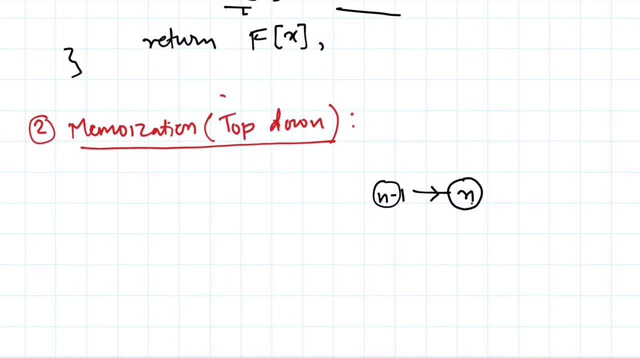 state n states from where we can reach here. so it will look at the state transition rule and it sees that I can reach to state n only from state n-1. so it will ask this state that what is your value? please tell me your value, then I can update my own value. so, but this state 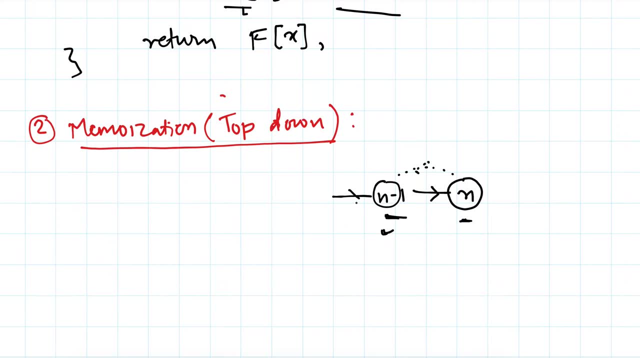 has not been solved yet. so what it will do? it will ask its previous state from where we can reach to this state. it will ask: I need your value to calculate my value. please send me your solution. so it will further ask n-2 until it reaches base 0 or the base state. 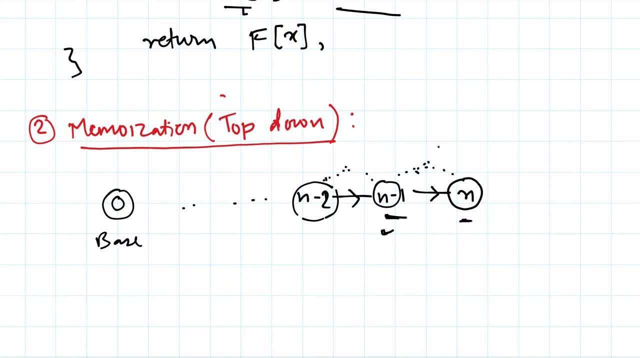 so we make recursive calls. This calls Some function f. we call this function fn. it calls fn-1. in turn it calls fn-2, until it reaches the base case where we will give some value and this function f0, will terminate. and now we will move to the stack of f1. then f1 will have value because f0 is there. so 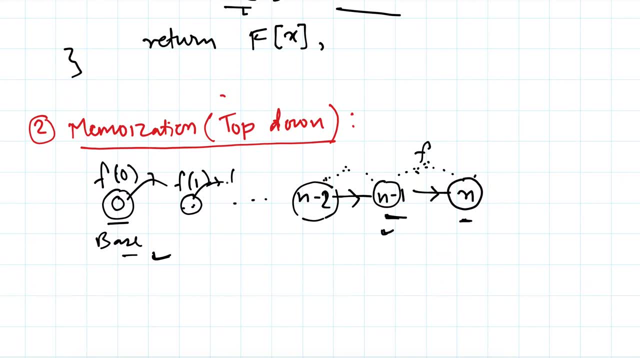 it will return back the value to the calling function f2.. So and then Then this function will unroll itself. so we had a sequence of call fn, fn-1, fn-2 till 210, so we had so many recursive calls. now it will start getting its value and start terminating. 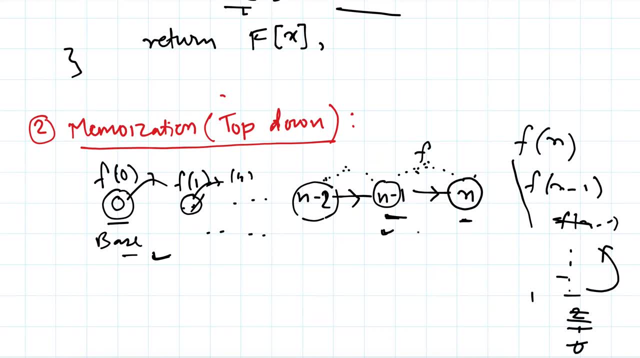 and returning its value to previous calling function. So here we started from the top state So And recursively reached the base state. so this is kind of top down approach. so instead of starting from the base state, we ask the answer from states that reach that destination. 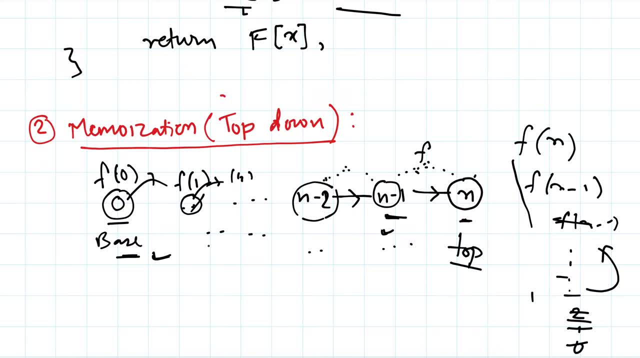 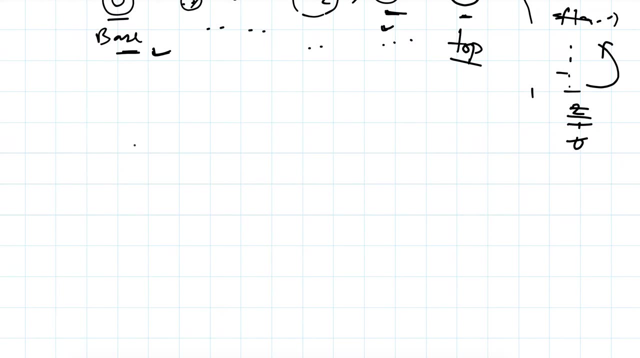 state. as for the state transition relationship, So start from top destination and compute its answer by taking in the value of states that can reach the destination state. So for the understanding purpose we can take some other example. this was one dimensional case, but we can have more practical example, like we have a graph, and this is the starting. 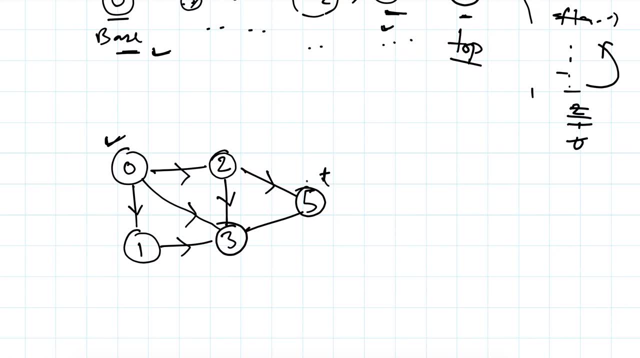 point. This is the destination point: source and destination. So I want to find the shortest path from zero to five. So in bottom up, what will we do? we will see. this is a starting point. so where else can I reach from this state? so I know that from here I can either go to two, three or one, so I will find the solution from. 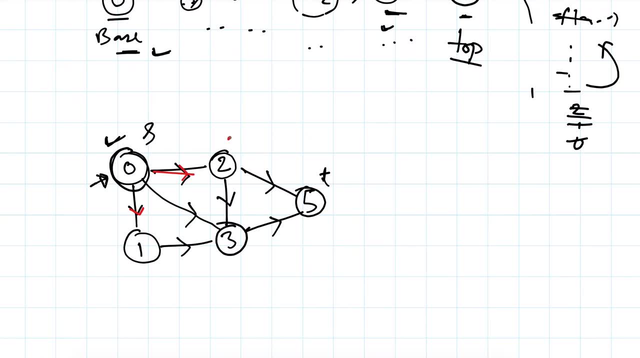 this 2 to 5, that is, our source has shifted, so we know that from source I can go to only 3 places. so if I know what is the shortest distance, from 2 to that destination, or 3 to that destination or 1 to that destination, then we will know the shortest distance from 0. similarly, 2 will. 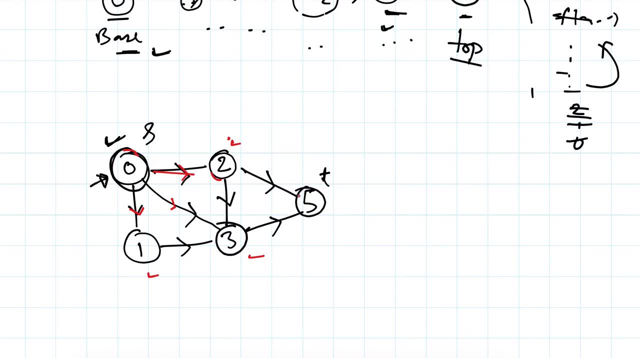 once we have the values for these, we can move ahead and this top down. what will it do? it will ask 2 and 5, 2 and 3, so it knows that we can reach 5 only from 3 or 2. there is no. 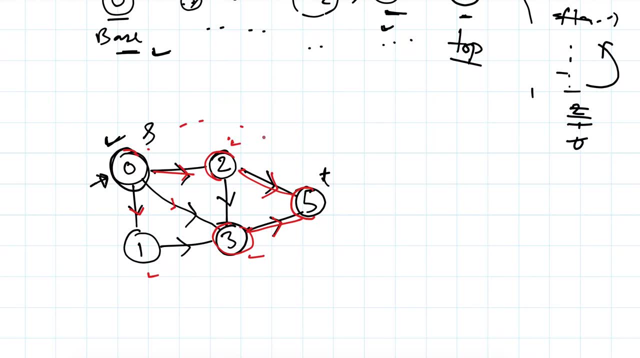 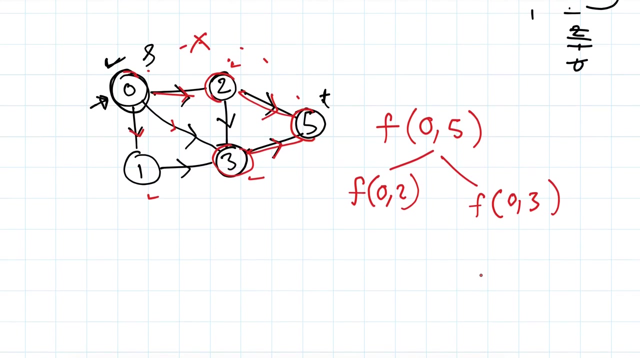 other way. we cannot directly go from 0 to 5. this is not possible. so now, if you have to solve for 0 to 5, we know that there is only 2 possibilities. if we can find 0 to 2 or 0 to 3, then we can easily find. 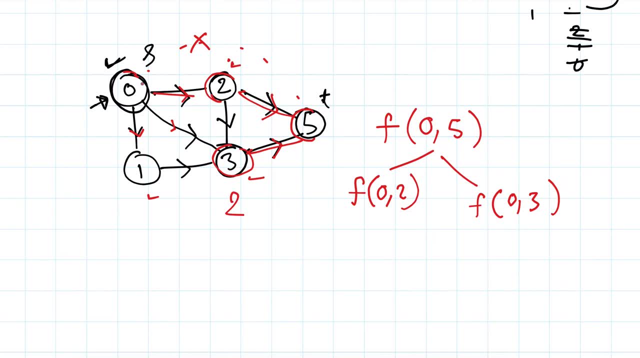 If shortest path form 0 to 3 is 2 and from 0 to 2 is 1, so it returns 2, it returns 1 and returns two. and now i see that these are neighboring. of these, the destination node that is, we can reach. 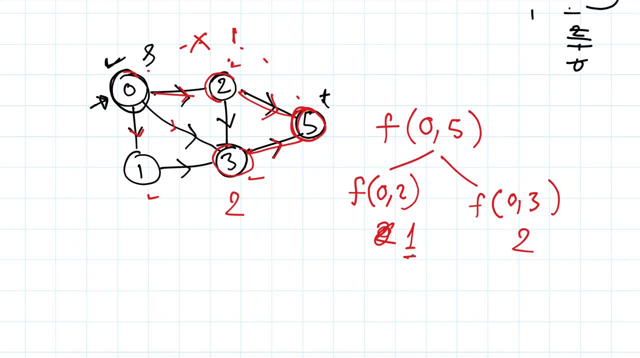 only from two or three, then we will pick whichever is minimum. one is minimum, so i know that it will return its value and add one to it, because there is one edge between that. so we will see that there is one path of a length three and one path of length two, so i will pick the minimum. so if i solve this for 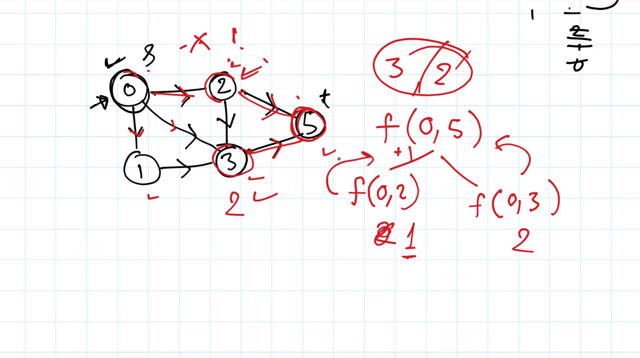 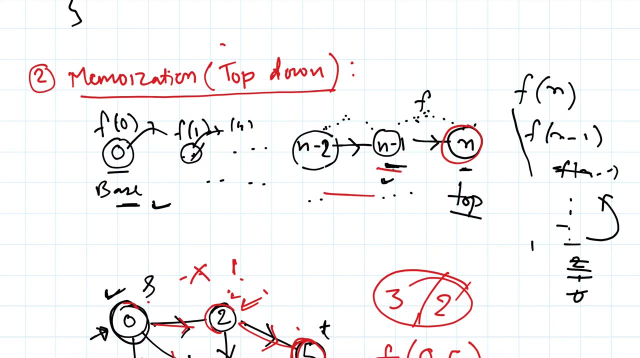 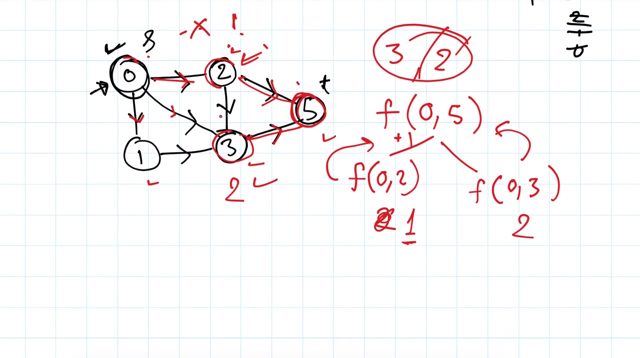 this node and this node we can solve for this node. so this is top down approach, just like this. so this state n ask its value from the previous state, and if this in turn asks its value from previous state, and so on till we reach the base state. so now i will write the same. 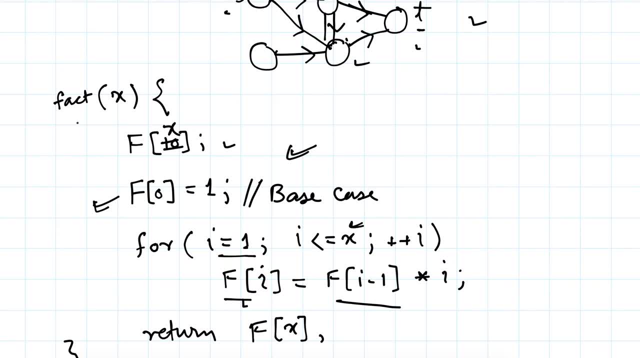 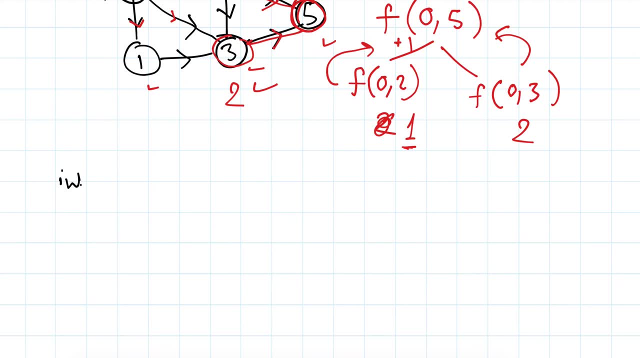 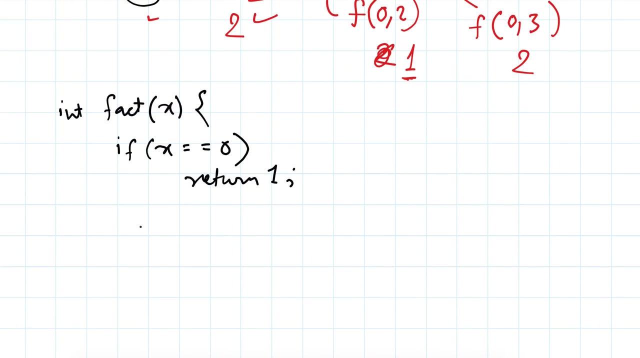 uh function factorial in the top down fashion. if x is 0, return 1 and we will keep one array to store the values, like earlier, because we need to store the values, otherwise we will have to resolve the problem. so this is the array we will be using to store the values. 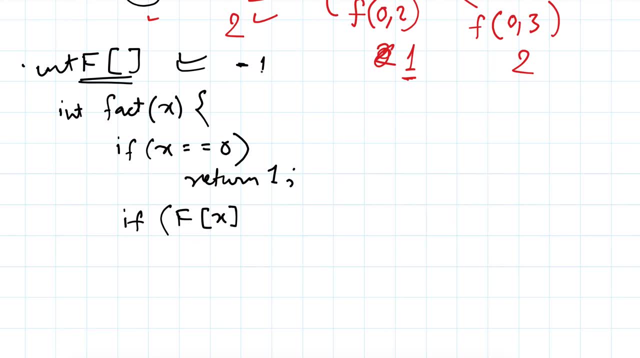 and maybe we can initialize it with some value, so negative factor, real or positive, so we can store negative values and first time we store the value it will become positive at that index and we will know that we don't need to solve this part. so if f, x is not equal to minus 1, that is, we have solved this earlier for this value of x. 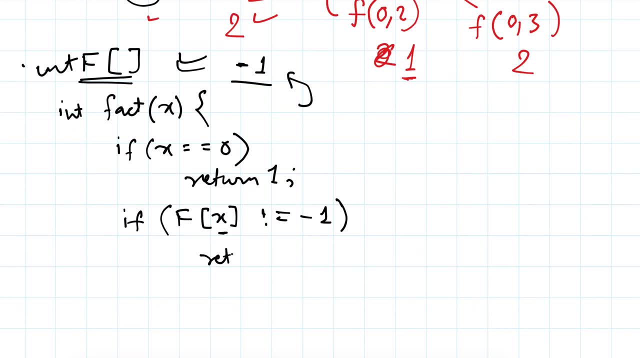 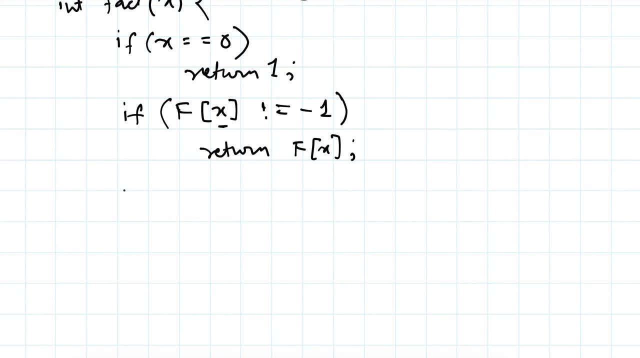 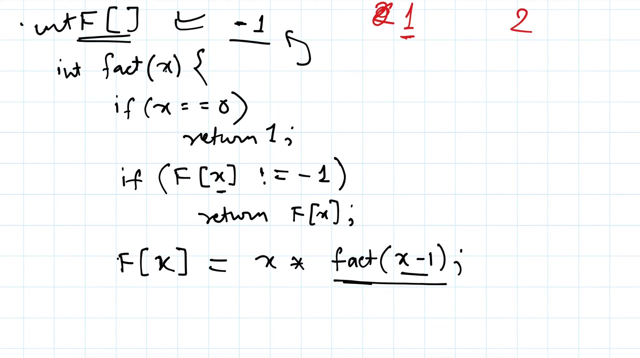 and we can use that value. so just return f of x. but if it was minus 1, that means we have not solved that problem before, so we will go ahead and solve that. so it will call that same function on x minus 1. so we call any call to function x. 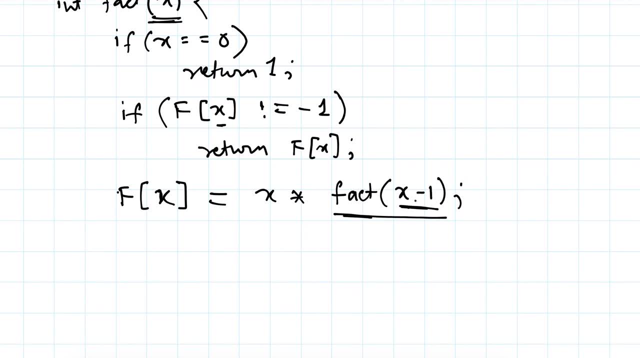 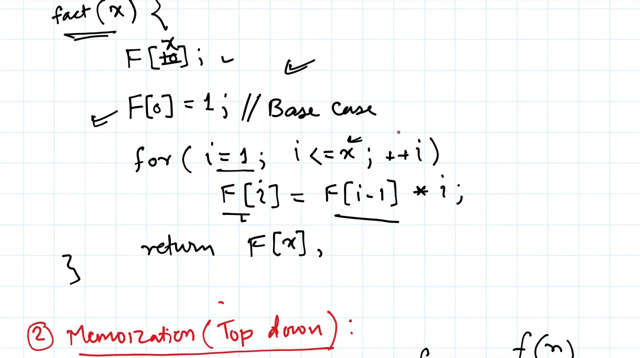 will call ultimately x minus 1, if it has not been solved earlier, and then store that value in f array and return that value. so we can see the difference in the two approaches. so in the top down we were calculating it using the value stored in array, because we are moving from the base case, so we will. we are. 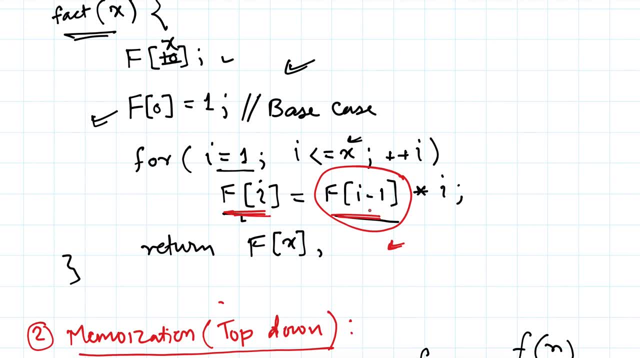 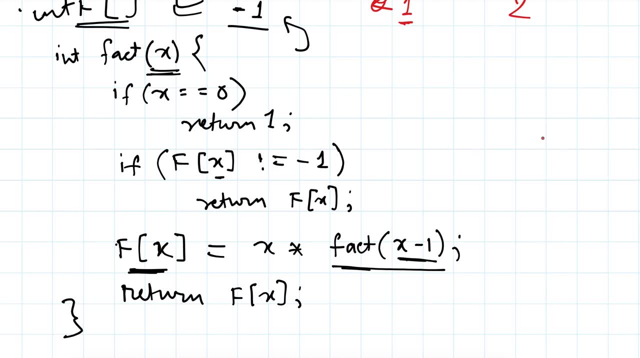 guaranteed to have the values in the array, this array, but here we are not sure whether the value is present or not, because we are moving from top to the bottom and top depends on that, so bottom, which has not been explored yet. so we first check if it has been solved or not. 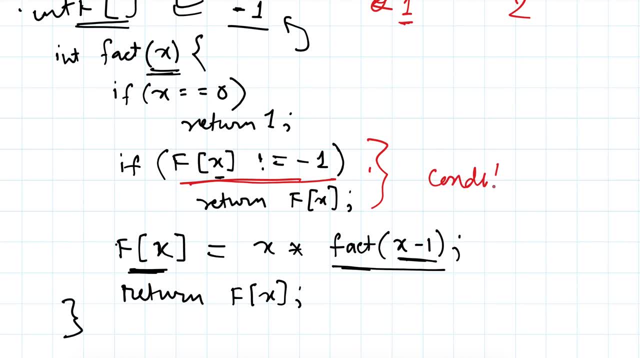 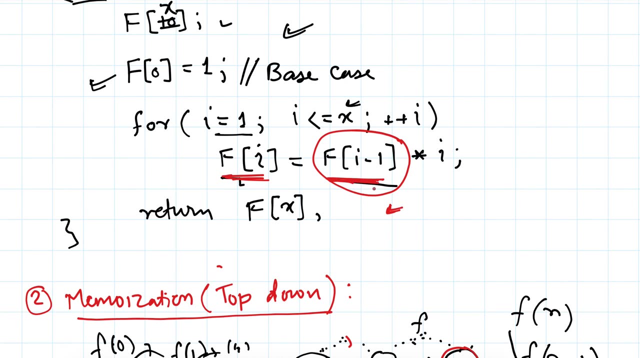 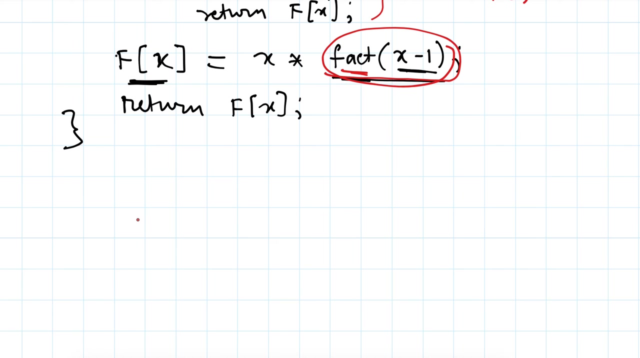 so this extra condition is here, which was not present in the bottom up, and here we have the recursive call. the same function called on lower state. here we did not have any recursive call, we were directly using the value from the table. so if we know that all sub problems must, 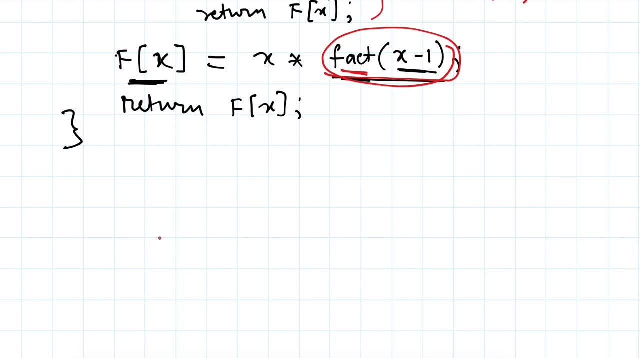 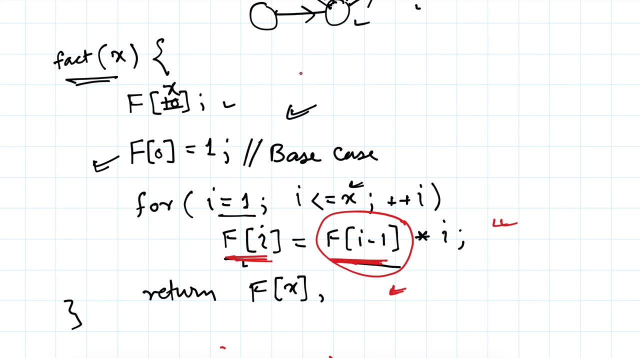 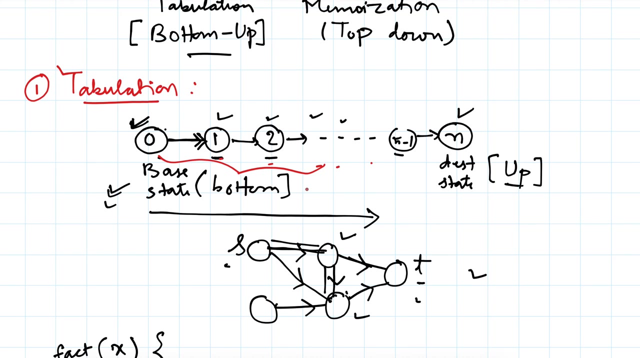 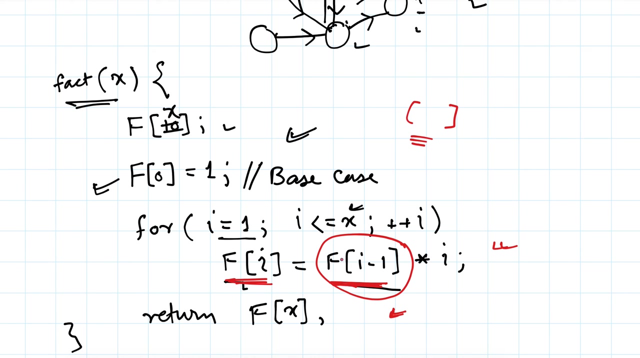 be solved at least once. then the bottom-up approach will work much faster because we are not doing any redundant calculation. all these base states values are required and and will be solved at least once. so we are not doing any redundant calculation and we are storing these values in some array and when required, we are directly whenever we call this function it. 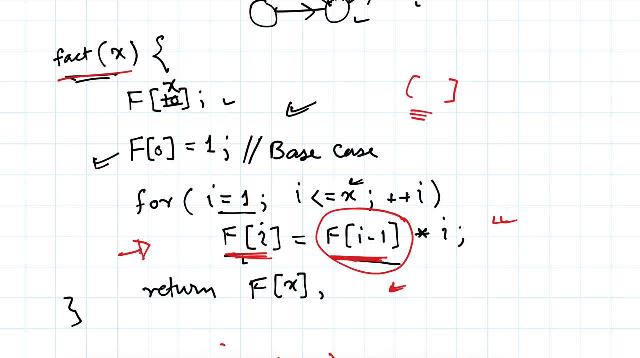 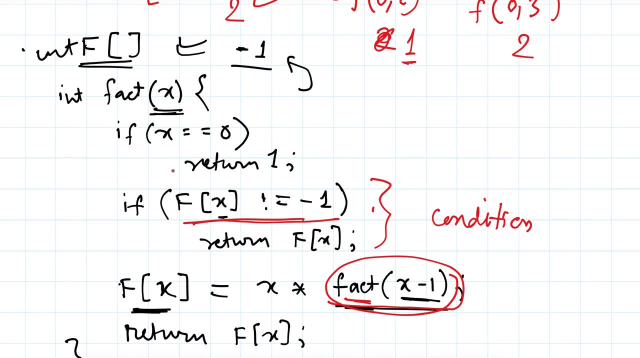 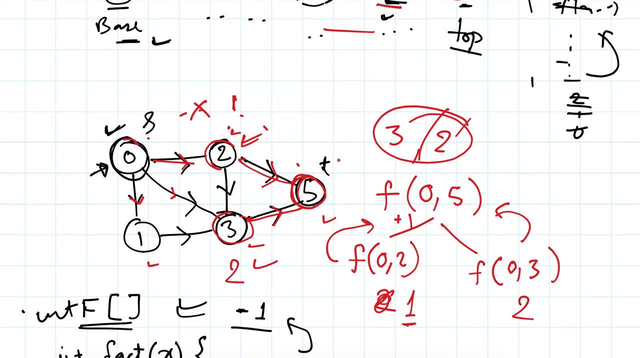 just need to access the array and return the value, whereas in this case it will do a recursive call of the same function with lower state and there will be too many nested recursive calls. so you? the first approach is supposed to be faster if we need to solve all the problems, but there. 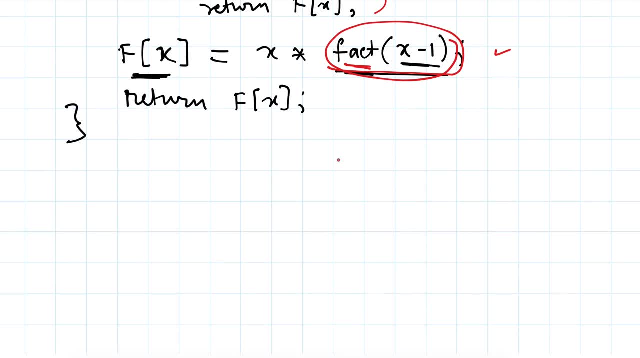 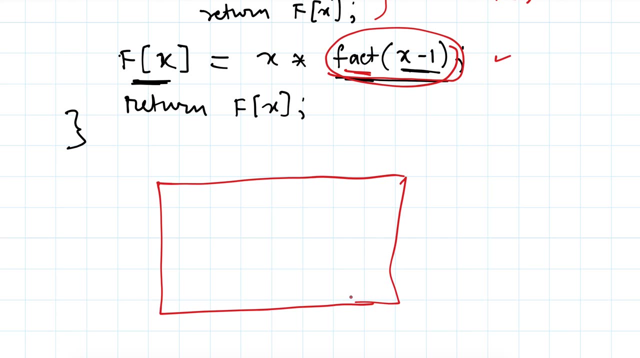 may be cases where we just need a subset of problems to be solved. in that case the top-down approach may perform better, like we are restoring some value in some 2d array, or maybe we can make it more complex 3d, 4d array and for calculation we have the way of calculating the 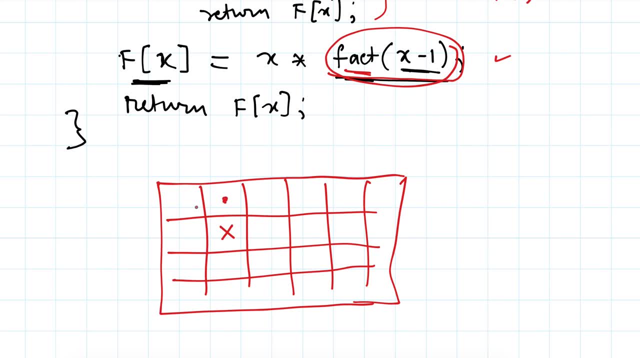 this value, we need the value of this cell and this cell, and then we move to next cell and for calculating this we will need only this and this and then we will reach here and we will need this and this value and this will be our required destination state. then we need to just solve for these values. but if we 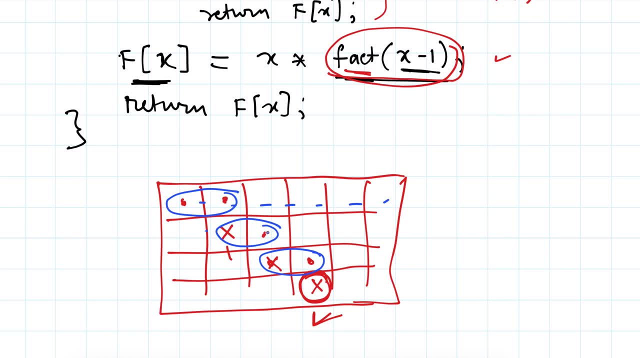 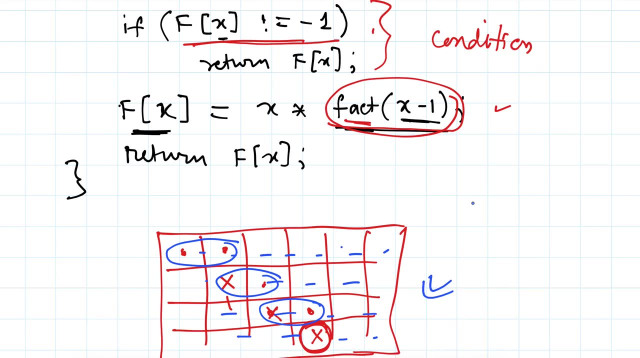 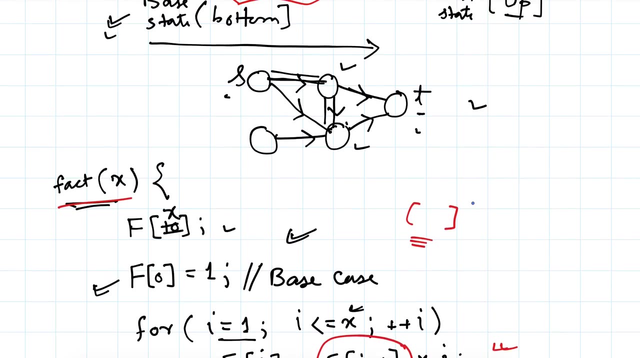 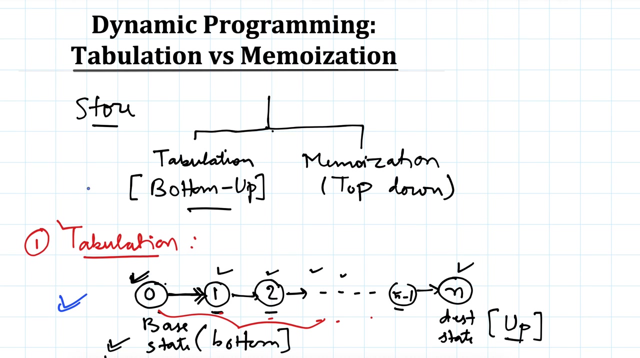 start from tabulation and start filling every value, then some calculations may be redundant in some cases, but if all sub problems need to be solved at least once, then we should use this bottom-up approach, and because it should be faster. so thanks for watching and those were the two main approaches for storing. 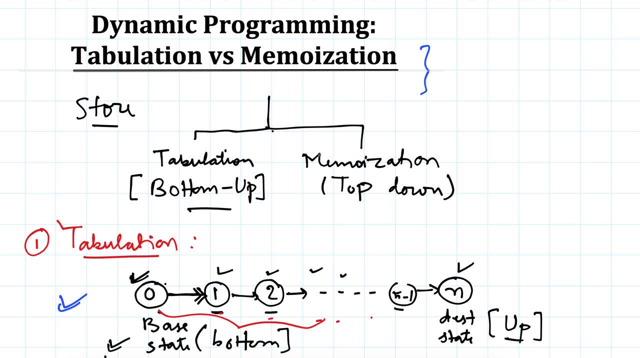 persisting the value of the cell. Please share your valuable feedback with me on in the comment section below and subscribe to my channel if you find it useful. thank you.